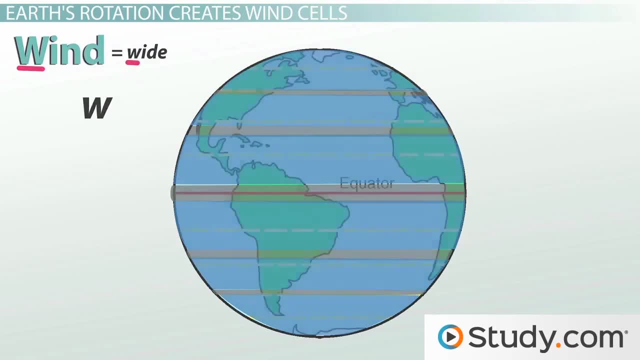 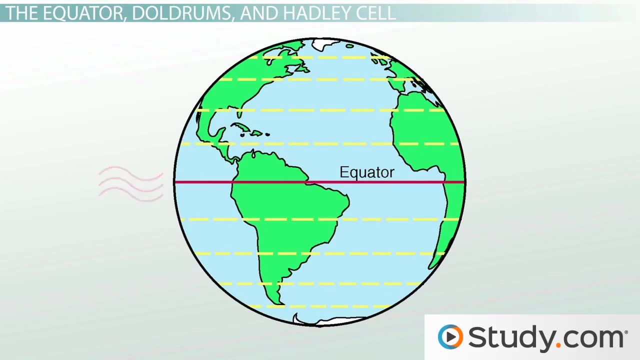 the windy cells are wide and both begin with W. Let's start along the equator. As you might expect, the air is very warm here, so it rises straight up. When warm air rises like this, it leaves behind an area of low pressure. You can remember. 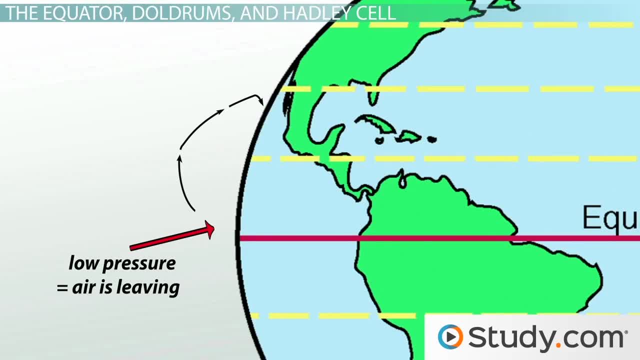 this because the air is leaving, which creates an area of low pressure, Leaving and low both begin with L. This particular area of low pressure along the equator is where we find our doldrums, a long stretch of stagnant air and our first windless strip between cells: The warm air. 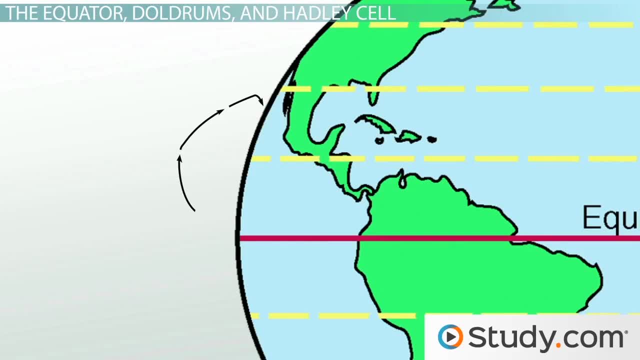 rising from the equator also brings a lot of moisture with it, and as the air rises it cools. The water in the air is pushed out and comes back down as rain. It's certainly no accident that we find the world's tropical rainforest along the equator. This is where 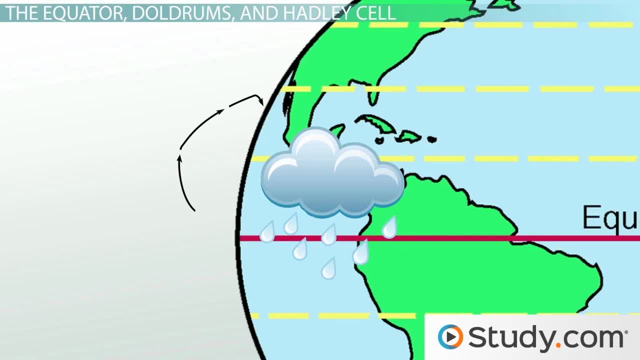 all that moisture from the hot equatorial air gets released. The warm air rising from the equator eventually begins to spread horizontally, which creates those wide, windy circulation cells. On either side of the doldrums are the Hadley cells, one for your hemisphere. 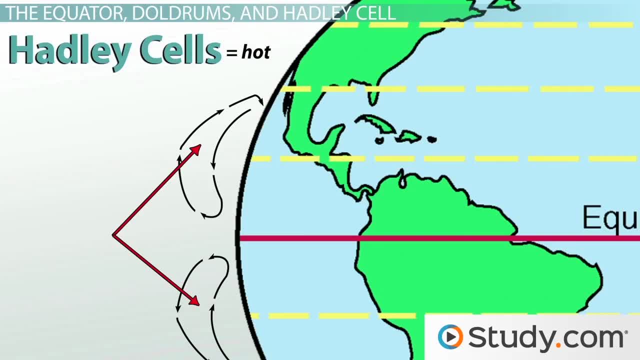 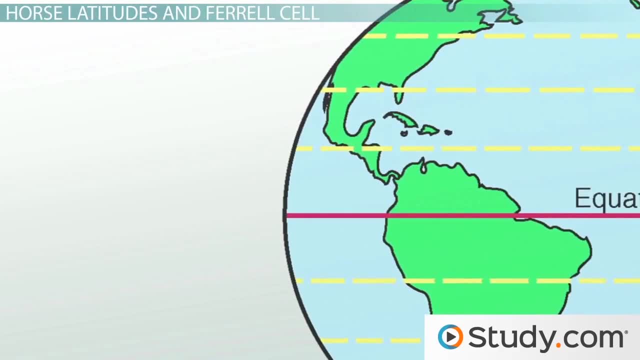 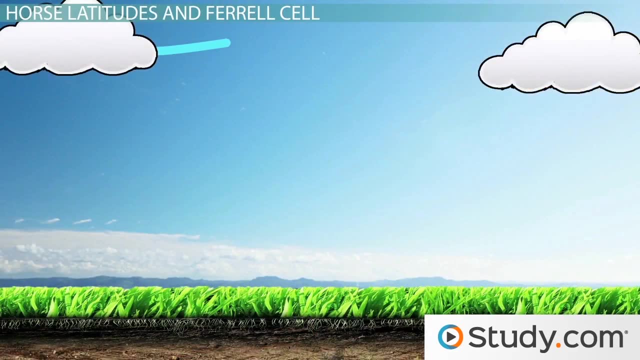 You can remember, the Hadley cell borders the equator, because the equator is hot and hot and Hadley both begin with H. As the air spreads horizontally, we find that it begins to cool even more around 30 degrees north and south latitudes. When the air is cool enough, it starts to fall back towards. 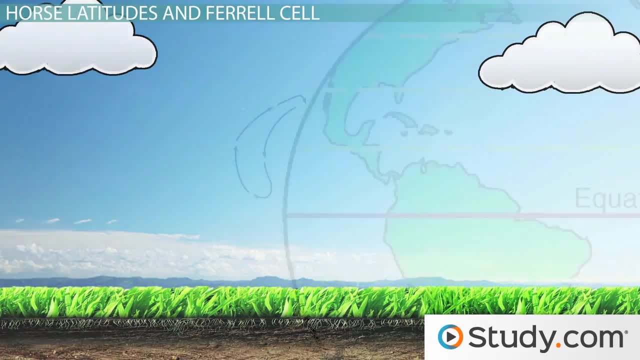 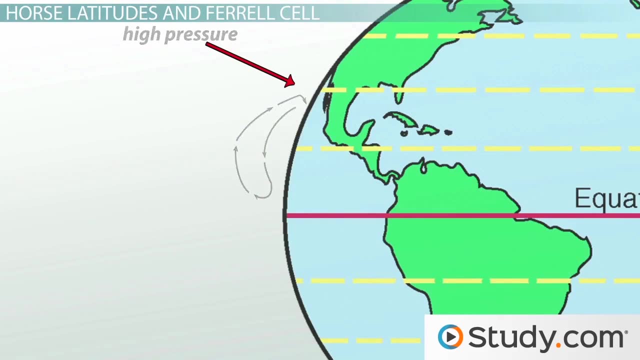 Earth's surface, but as it falls it warms. So if hot air leaving creates low pressure, hot air coming in creates the opposite: high pressure. Because of this, the falling air creates our next thin, windless strip called the horse. 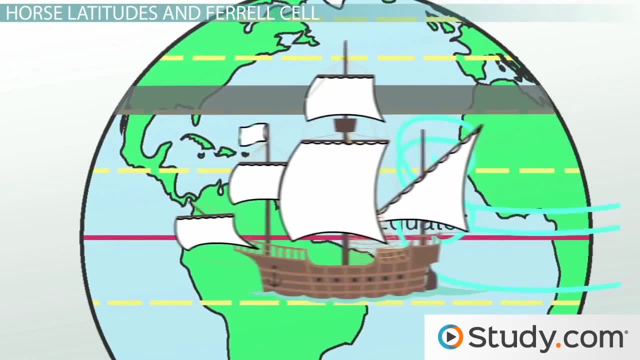 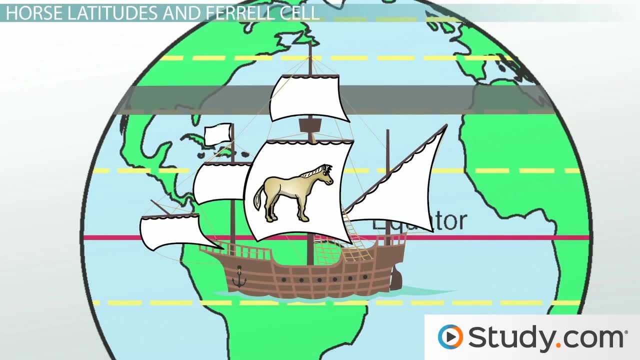 latitudes. They were named this because, like the doldrums, there is little wind to push ships along the ocean. Legend has it that when this happened, horses on board the ship were either eaten, as food supplies went low, or thrown overboard to reduce the load. The 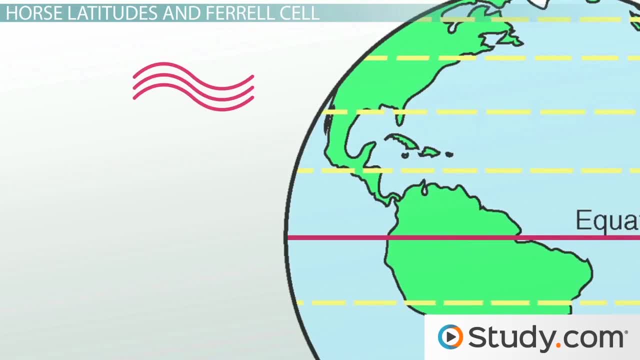 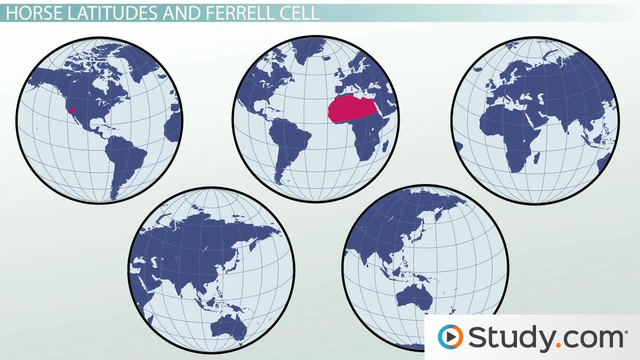 horse latitudes create areas of hot, dry surface air around Earth. You might not be surprised to learn that this is also where we find the world's most important natural resources: the world's great deserts like the Sahara in Africa, the Mojave in the US and the Great 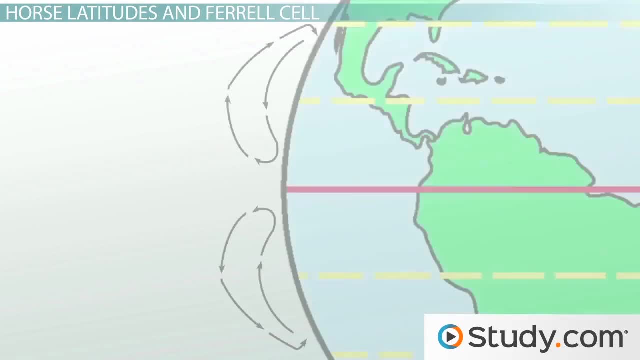 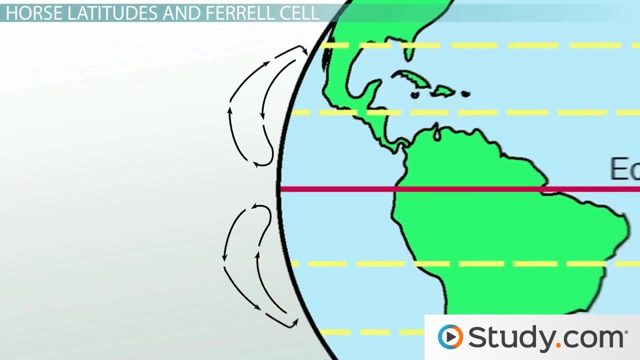 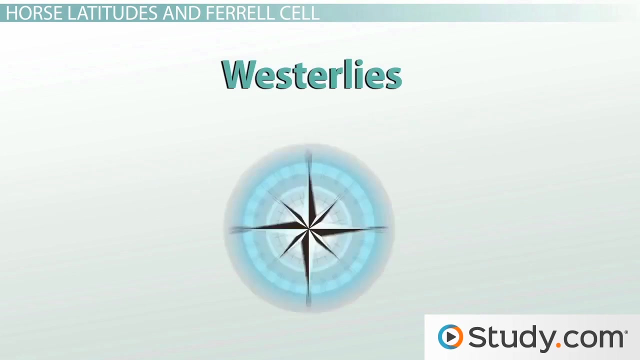 Victoria in Australia. Some of the air heads back towards the equator as the warm, steady breezes of the trade winds, but much of it keeps heading towards the poles, creating our next cell, the ferrule cell. The winds that blow towards the poles and create the ferrule cells are the westerlies. 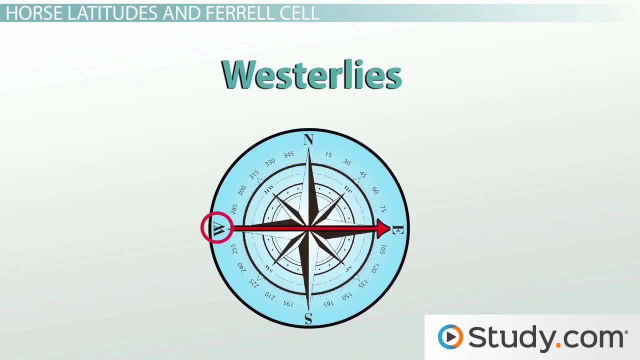 which you can remember, because they come from the west and blow to the east. When the warm, moist air that comes from the west and the western wind that comes from the north and the south blows towards the east, we find that the wind that blows towards the 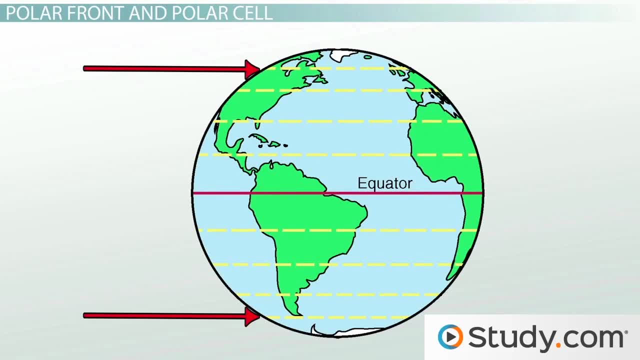 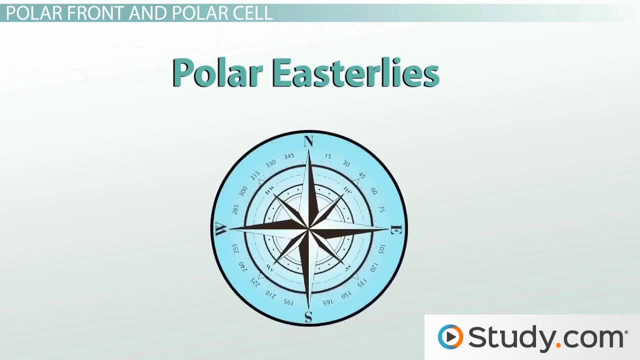 west is called the ferrule cell. When the warm, moist air that comes from the north and the western wind, These westerlies reach about 60 degrees north and south, twice the latitude as our other thin, windless strip. They meet up with the cold, dry polar easterlies which, as you have probably guessed, blow 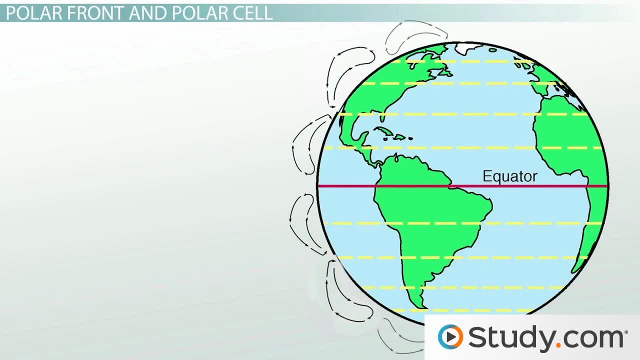 from the east. The polar easterlies make up our third and final circulation cell, the polar cell, And where the polar cell and the ferrule cell meet is called the polar front. Here, just like at the equator, air rises vertically and that leaving air creates an 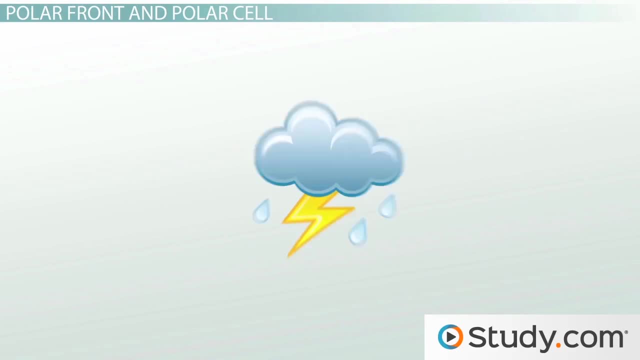 area of low pressure. The other interesting thing that these two different temperature cells create when they come together is storms. As we learned in another lesson, fronts are contact areas between two different air masses. When these air masses meet, they're so different that it's almost like they're fighting about. 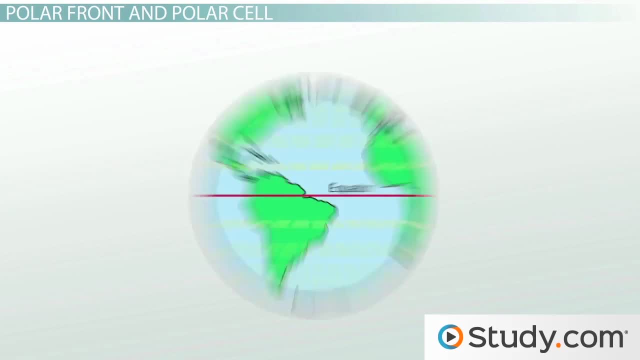 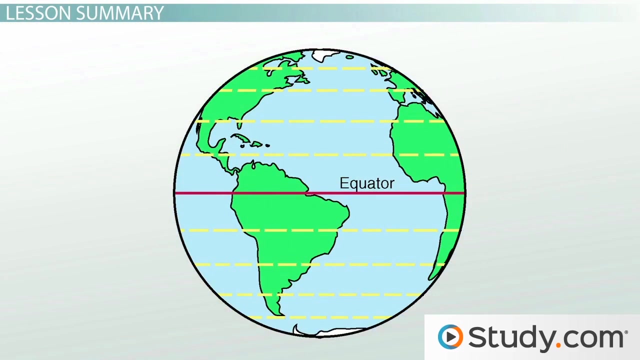 the weather and the storm is like they're conflict. The polar front is no exception, And these areas on Earth are well known for their unpredictable storms. Earth spins on its axis, which creates interesting wind patterns around Earth. Among these interesting patterns are global air circulation cells, three in the northern 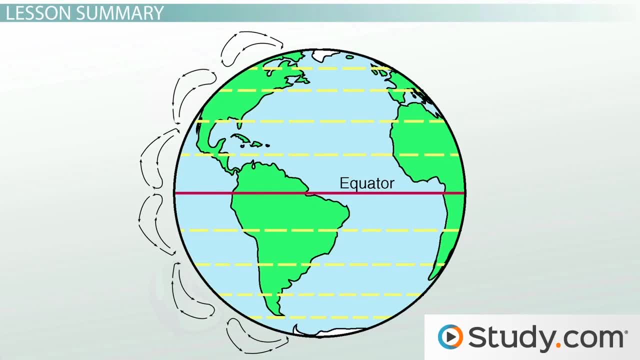 hemisphere and three in the southern hemisphere. These cells help distribute heat and air across Earth, as each cell is like a wide windy belt around the globe. Where each cell meets, another is also like a belt, but these are opposite to the one in the northern hemisphere. 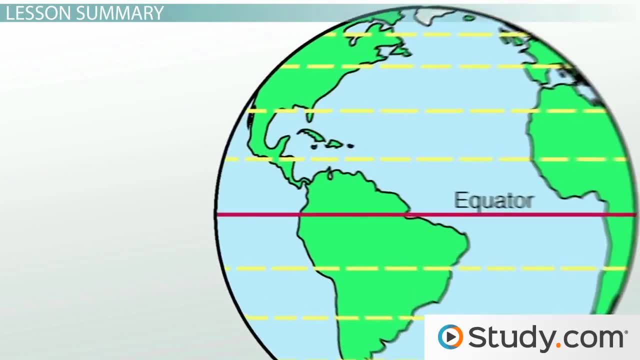 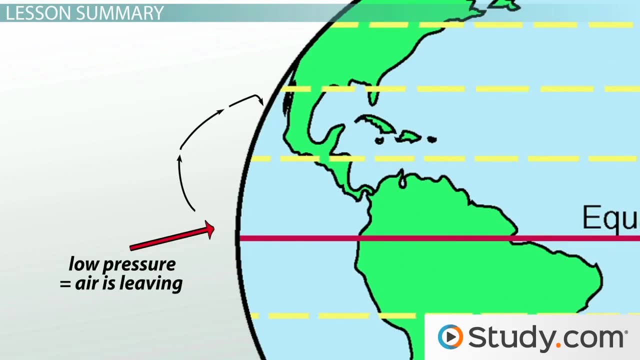 These cells are also called wind cells. These cells are also called wind cells acting like thin windless girdles. Warm air rises vertically along the equator and when that air leaves, it creates an area of low pressure. This is our first windless strip: the doldrums. 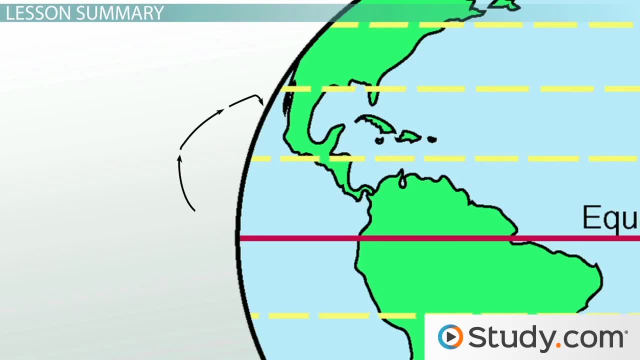 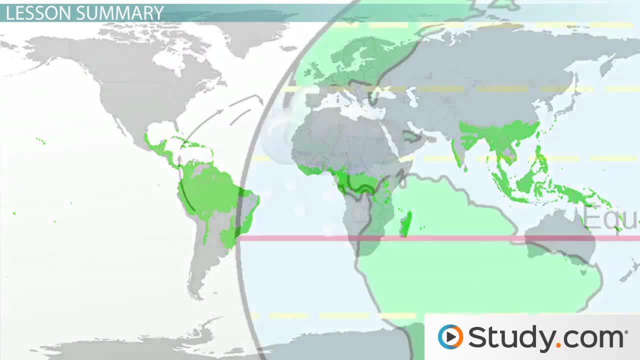 As the vertically rising air cools, it rains a lot of the ocean moisture it brought with it back down onto land, which is why we find the tropical rainforest in this area. At some point, the air starts traveling horizontally, creating the first cell, the Hadley's cell.